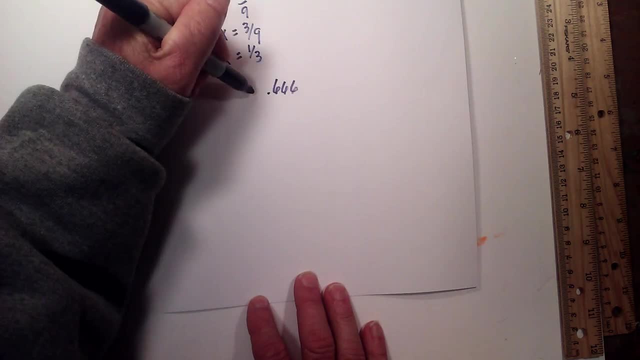 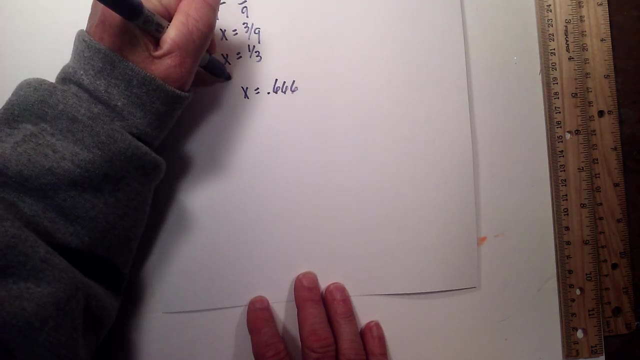 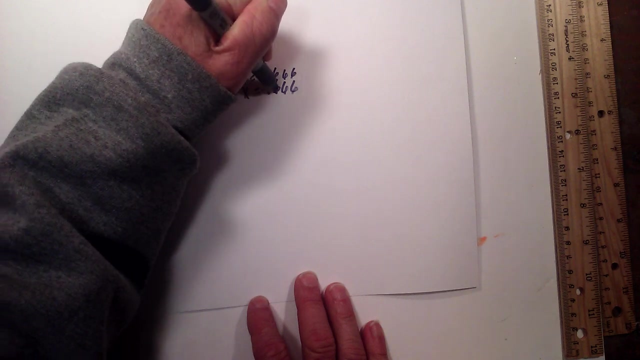 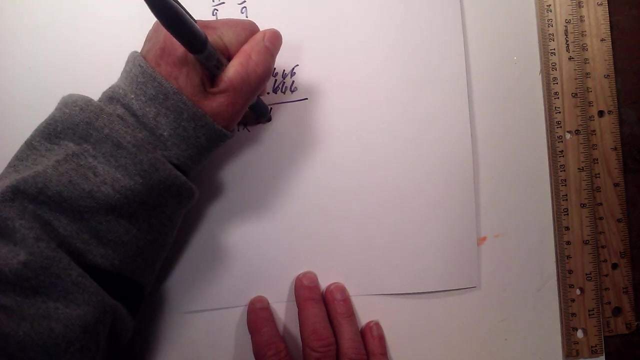 0.666, I'm going to set it to x. okay, I have one digit repeating, so I'm going to multiply it by 10, so this will be: 10x is equal to 6.666. these cancel subtract we have. 9x is equal to 6. 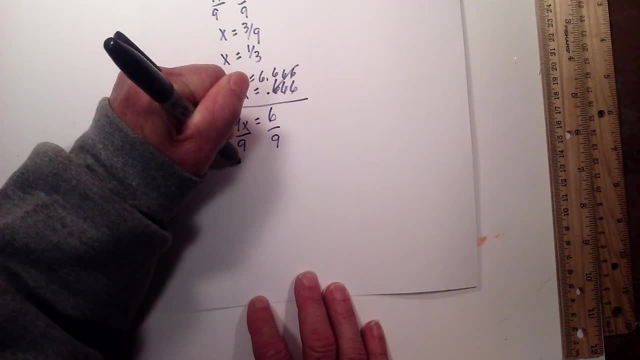 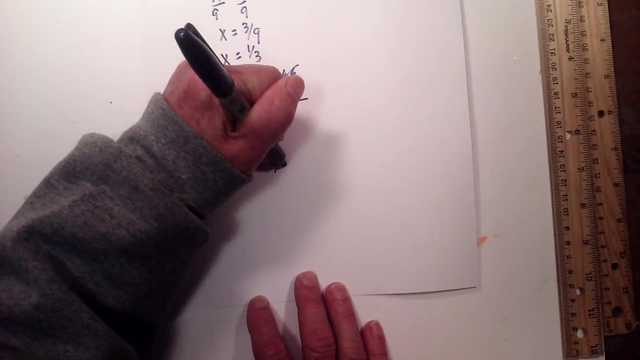 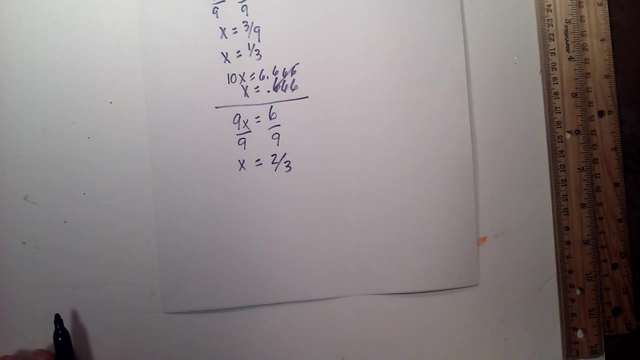 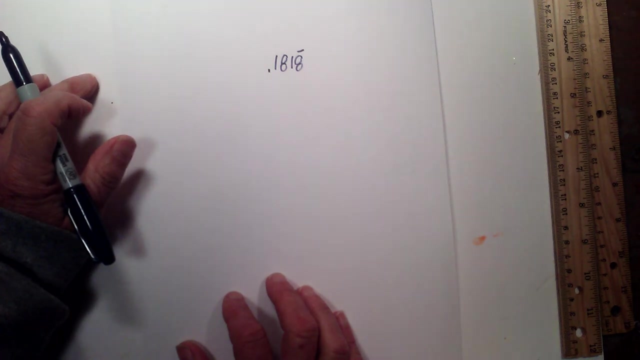 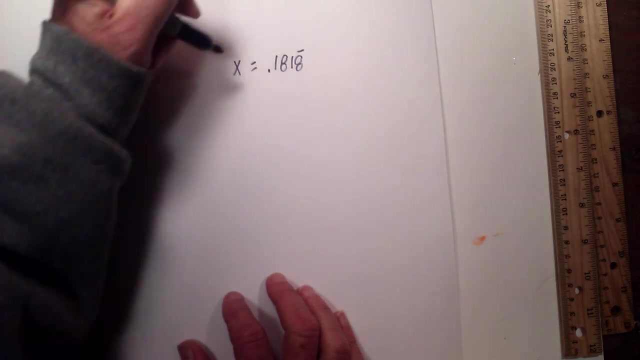 divide both sides by 9x is equal to, and then 3 will go into both of those two thirds. okay, so now what's What about if we get a number like this? What if it is a number 0.1818 repeating? What we can do again is set it to x. and now, since we have two digits repeating, we are. 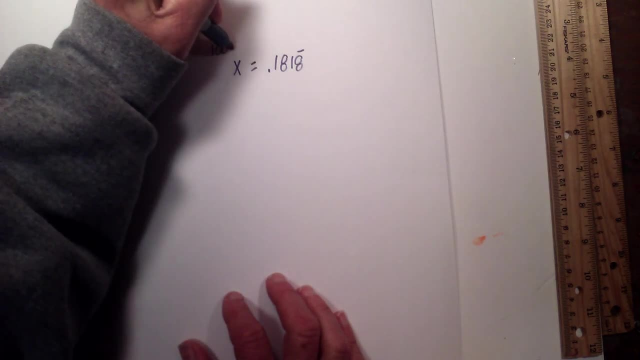 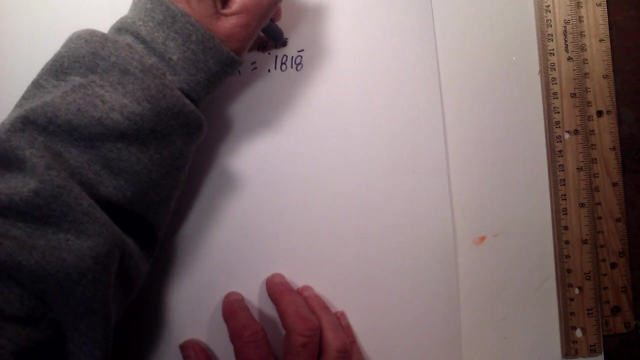 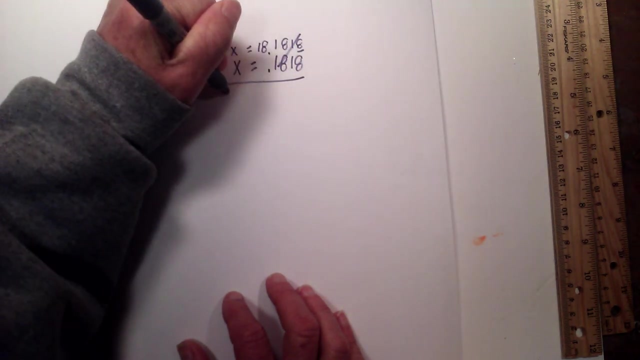 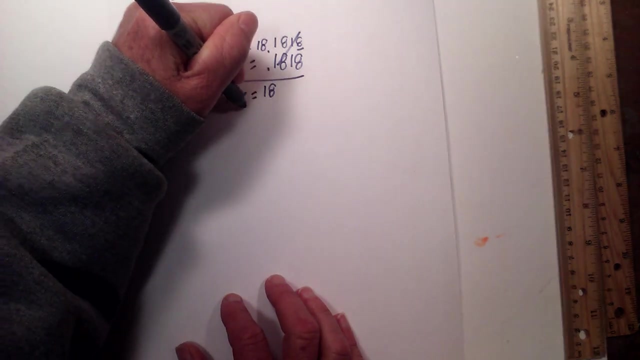 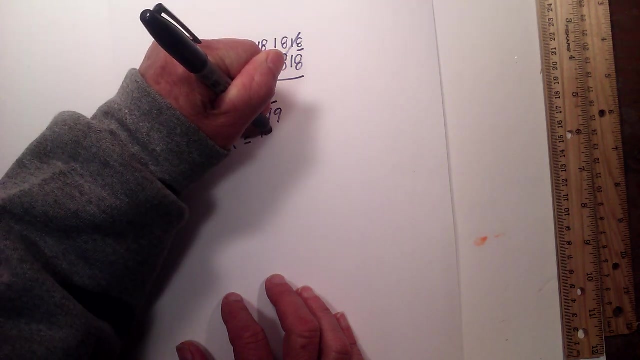 going to multiply by 100x. So 100x is equal to 18.1818.. All this cancels. We now have 99x is equal to 18.. Divide both sides by 99.. X is equal to 18 over 99.. 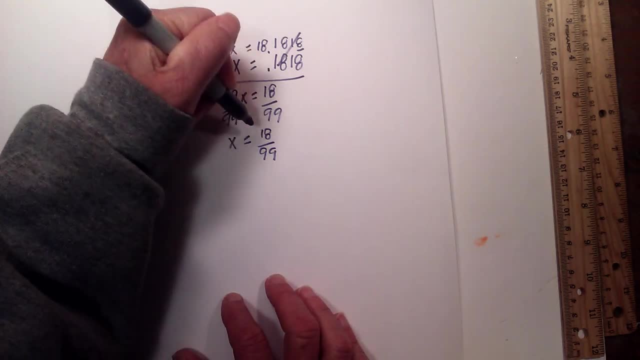 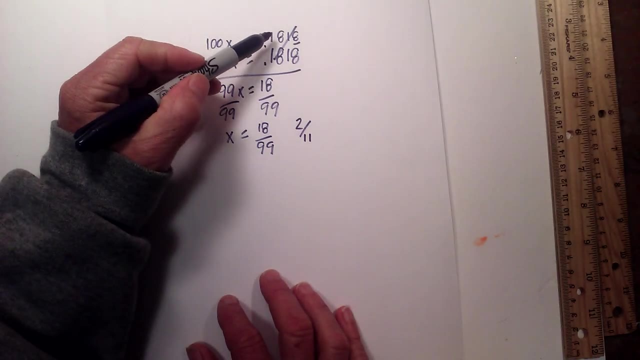 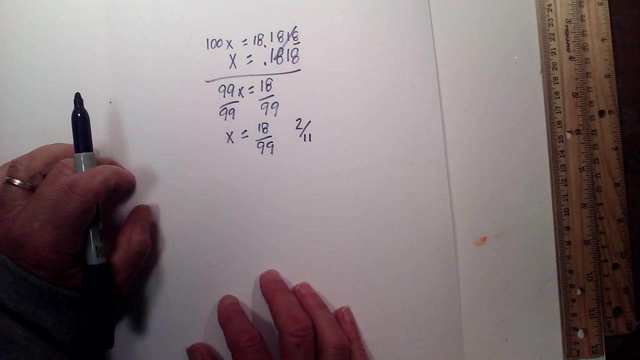 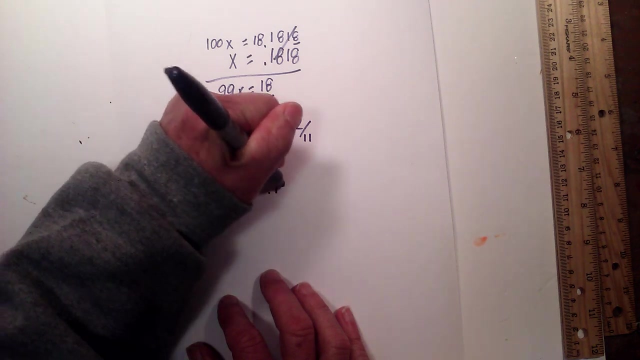 And then this can reduce down to 9 to 11.. So again, since we have two digits repeating, we will multiply it by 100 instead of 10x. Now, sometimes you will get something with a non-repeating number. What about if we have 0.166 repeating? 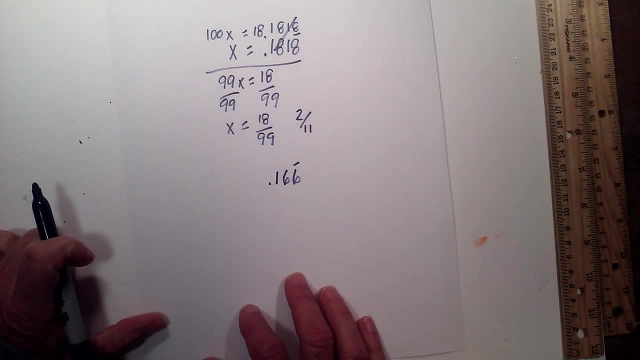 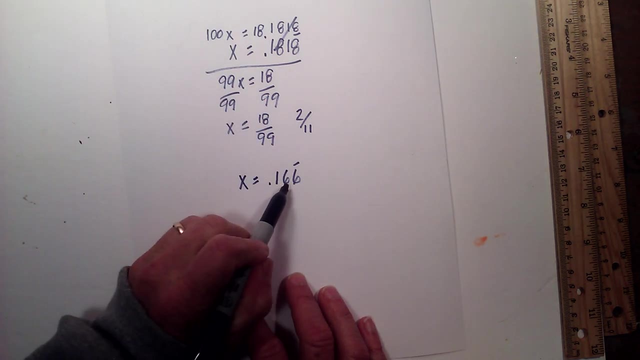 What are we going to do with this? Well, we are going to kind of do the same thing. We are going to set it to x. X is equal to 0.166.. But instead we do only have one digit repeating, but we have a non-repeating digit. 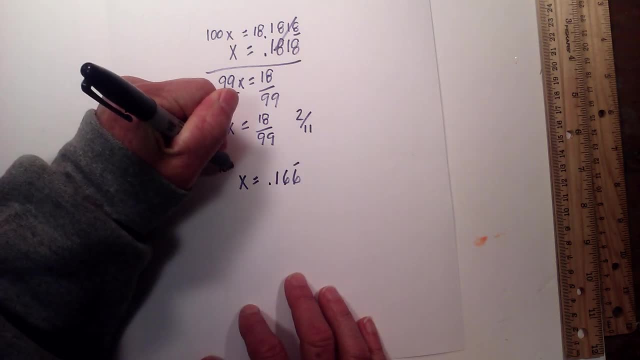 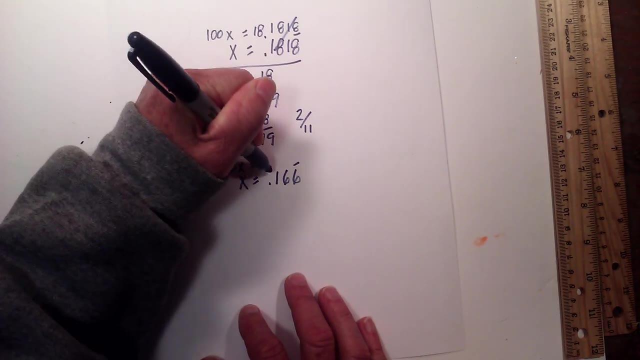 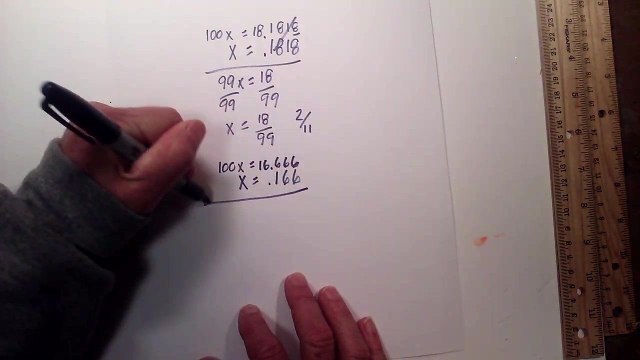 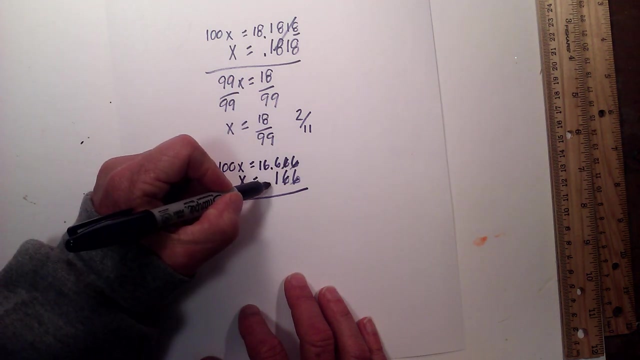 So instead of multiplying it by 10, we are going to multiply it by 100. again equals, And then now we are going to get 16.664.. Okay, So now it does not cancel out exactly like before. These cancel, But now we have 0.6 minus 1.. 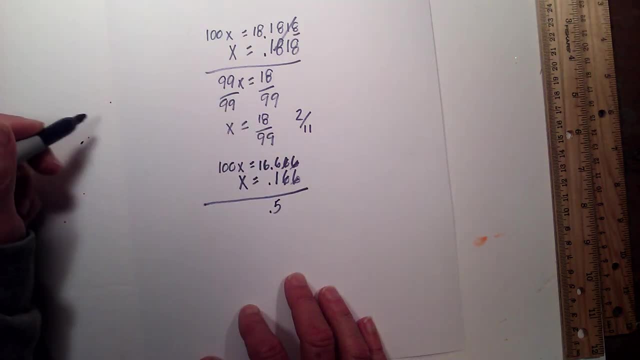 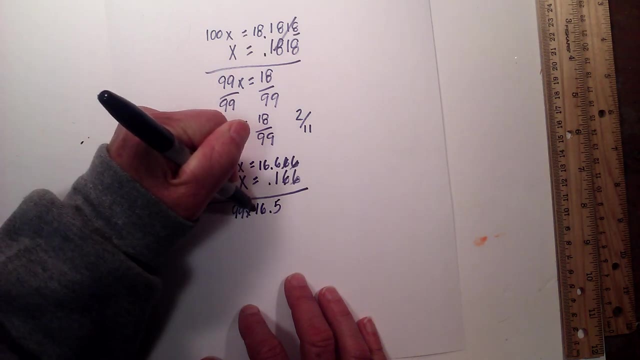 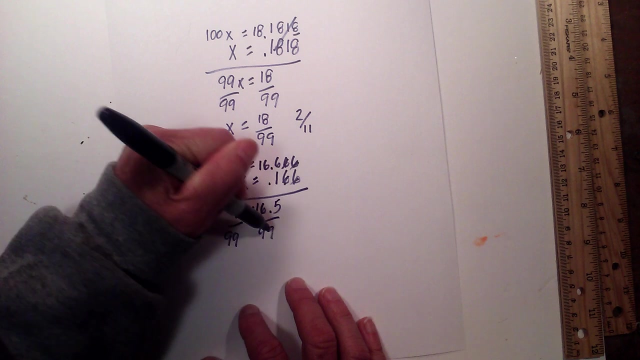 That will be 5.5.. Bring down the decimal when you subtract So you will have 16.5 is equal to 99x. It is kind of messy, So let's divide both sides by 99.. Okay, So x is equal to 16.5 over 99.. 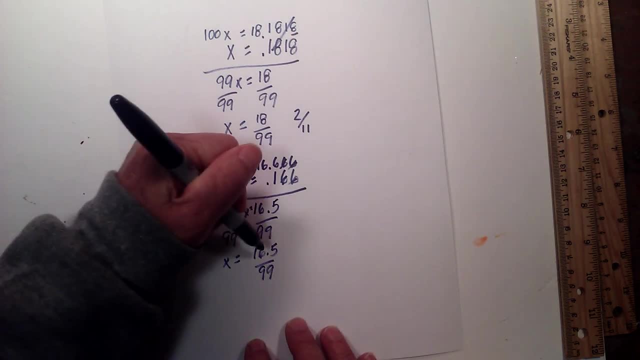 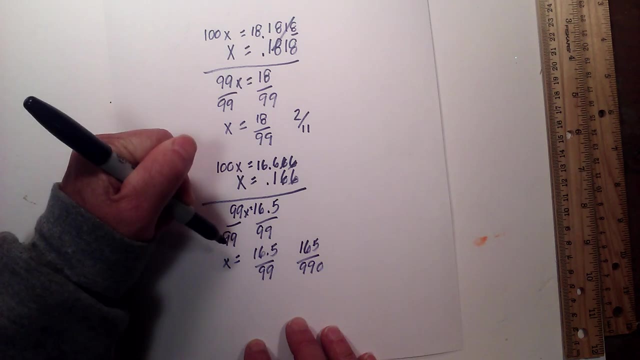 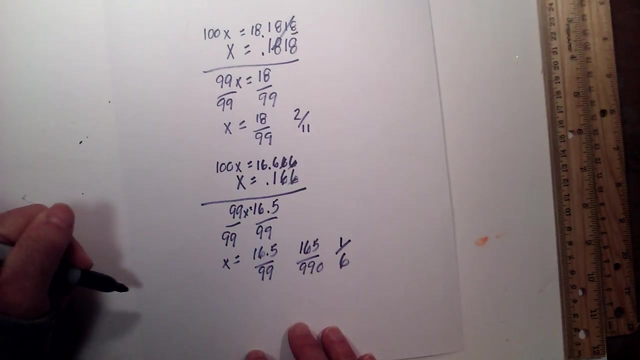 Now to get rid of the decimal, just multiply it by 10.. So this becomes 165 over 990.. And, believe it or not, 165 will go into 996 times, So it becomes 16.. So x is equal to 16.. 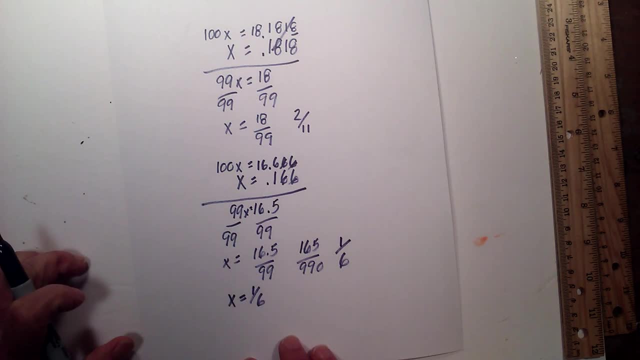 So I hope that helps in converting Repeating decimals into a fraction. Thanks for watching, and MooMooMath uploads a new math and science video every day. Please subscribe and share. 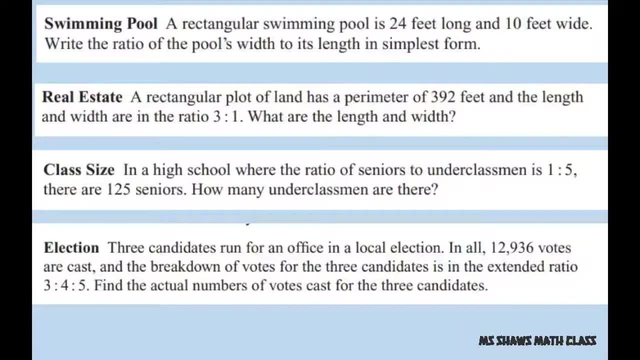 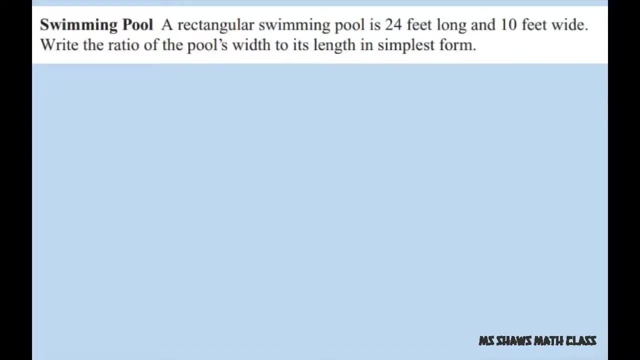 Hi everyone. we are doing four examples of ratio word problems in the real world and these are the four problems we're doing. The first problem, the swimming pool problem, is basically: it wants you to write the ratio of the pool's width to length in simplest form. Well, the width is 10 feet wide. 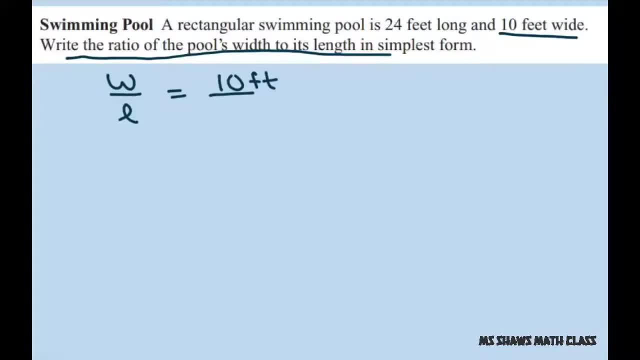 and so I'll put 10 feet, and the swimming pool is 24 feet, So they just want you to simplify this. So the feet cancel. We're left with 10 divided by 24.. What I'm going to do is divide each piece by.